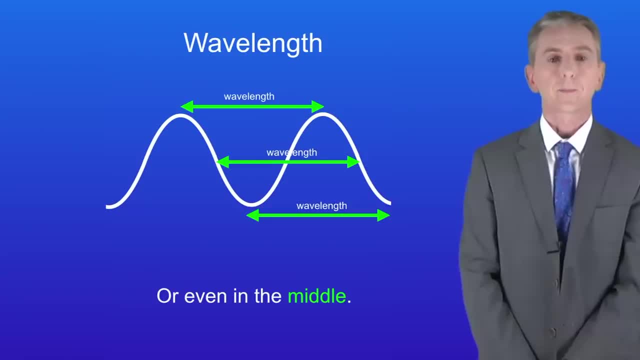 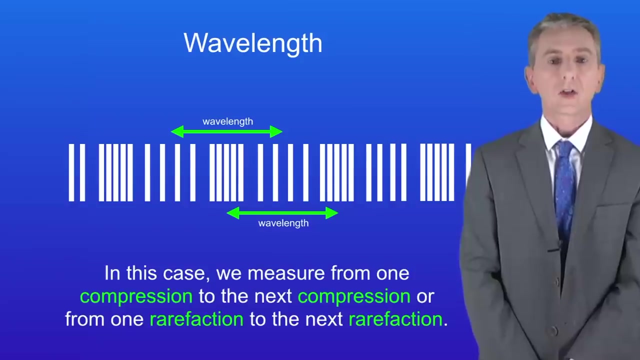 the bottom of the waves, like this, Or even in the middle, like this. Now, the wavelength has a special symbol, which I'm showing you here. This is the greek letter lambda, and we'll be seeing that again in the next video. Now we can also measure the wavelength on longitudinal waves. In this case, we measure from one compression to 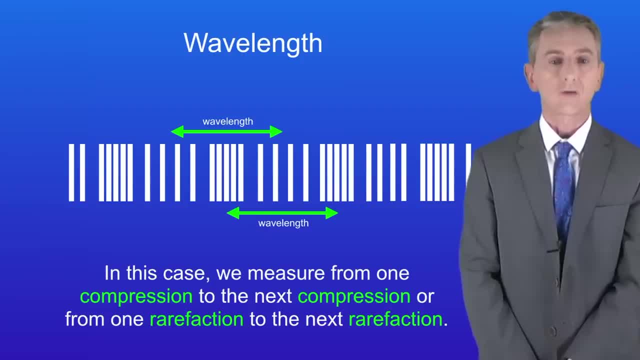 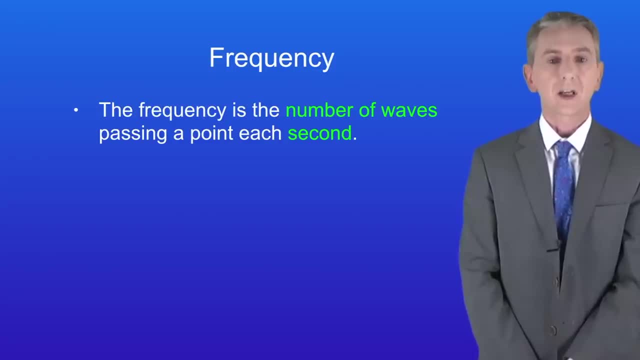 the next compression, or from one rarefaction to the next rarefaction. Okay, the next property of waves is the frequency. The frequency is the number of waves passing a point each second, and the unit of frequency is the hertz. One hertz equals one wave per second. 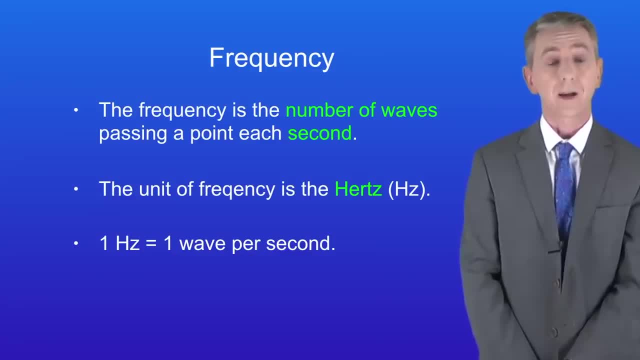 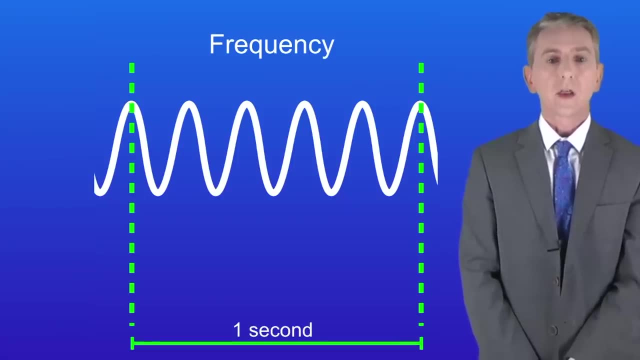 Now in the exam, you could be asked to work out the frequency of a wave from a diagram. So let's look at that now. Here's a transverse wave with the time shown on the bottom. You can see that this represents one second. 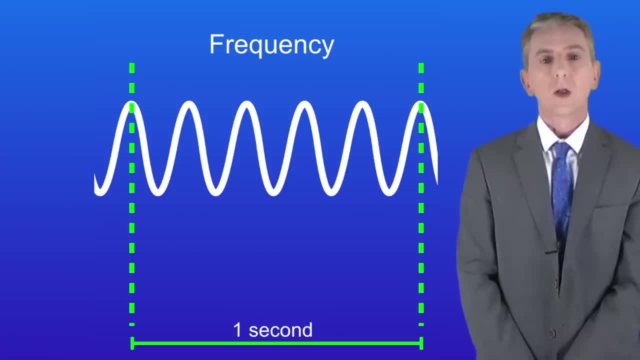 To work out the frequency we need to count the total number of waves. We can count one, two, three, four and five waves. So that means that the frequency is five waves per second, In other words five hertz. Here's another wave, and this one's got a longer wavelength. 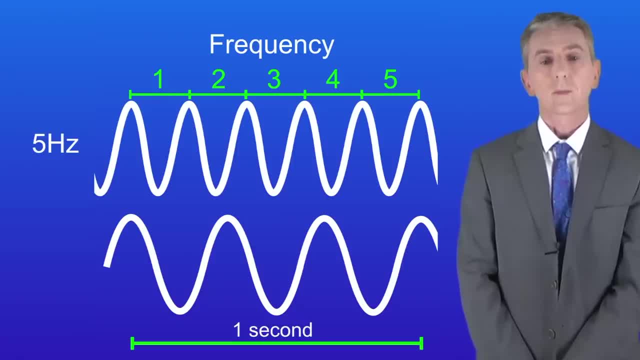 So again, to work out the frequency, we need to count the total number of waves. In this case we've got one, two and three waves in one second, So the frequency is three hertz. Now the final property of waves is called the period. 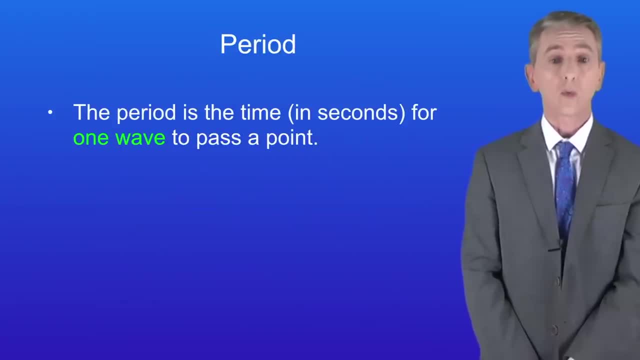 The period is the time in seconds for one wave to pass a point. We calculate the period using this equation. This is given to you in your exam, but the units are not given, so you need to learn them. The period in seconds equals one divided by the frequency in hertz. 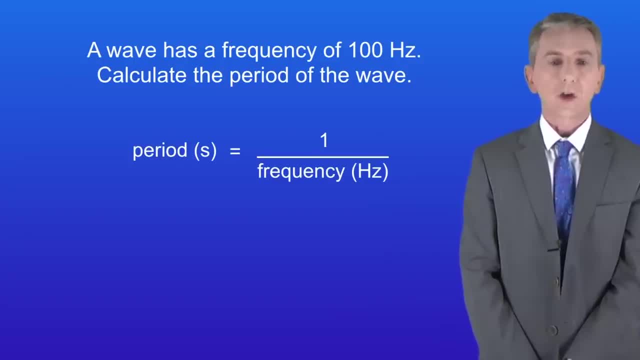 Here's a sample question for you. A wave has a frequency of 100 hertz. Calculate the period of the wave. So pause the video and try this yourself. Okay, so the period is one divided by the frequency. The frequency is 100 hertz. 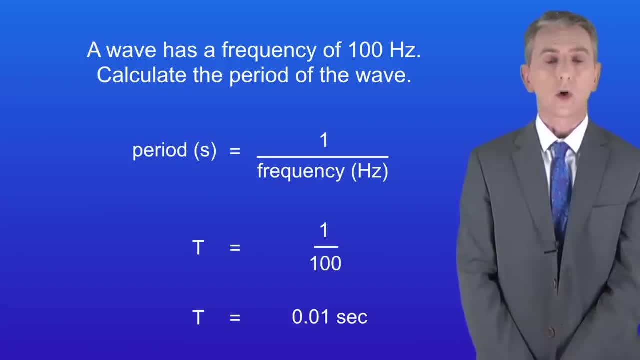 Dividing one by 100 gives us a period of 0.01 seconds. Remember, you'll find plenty of questions on the properties of waves in my revision workbook and you can get that by clicking on the link above.